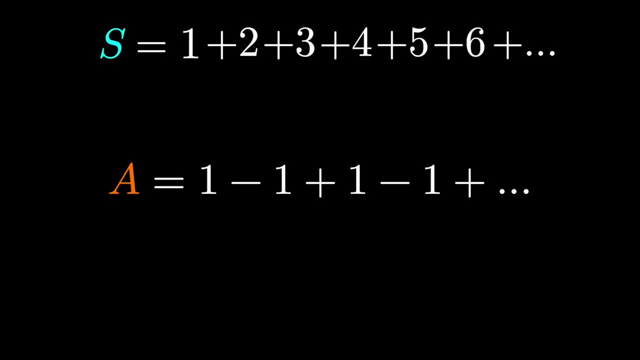 This is its own problem, but a quick way to go about dealing with this is to look at 1 minus a. That would be 1 minus 1 minus 1 plus 1 minus 1, so on forever. Just distribute this negative and this would be 1 minus 1 plus 1 minus 1 plus 1 minus 1. 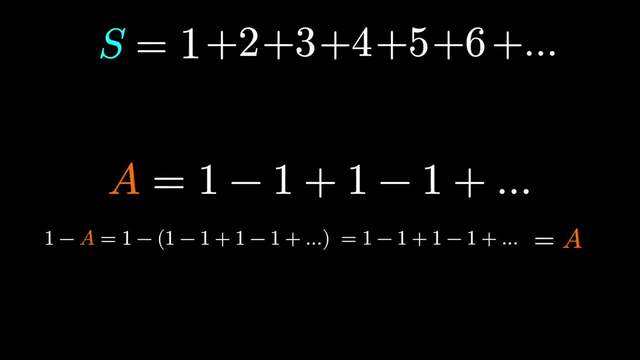 on forever. That's what we called a. So 1 minus a equals a, That's 1 equals 2a, Or a is 1 half. Now I can already feel you getting a little bit uncomfortable, but let's just keep going. 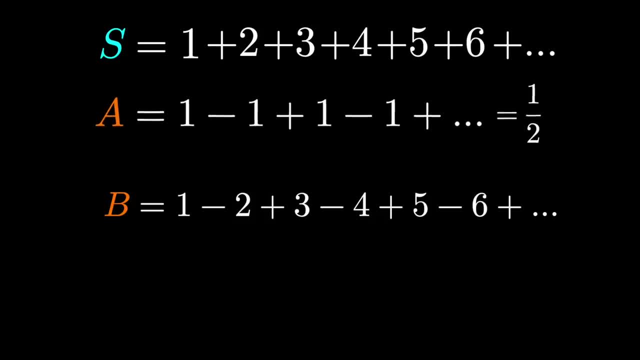 Here's what we'll call b. b is 1 minus 2 plus 3 minus 4 plus 5 minus 6, on and on forever. Not quite s, but we're getting closer. Add b to itself. Do it in a particular way where we shift all the terms over one space. 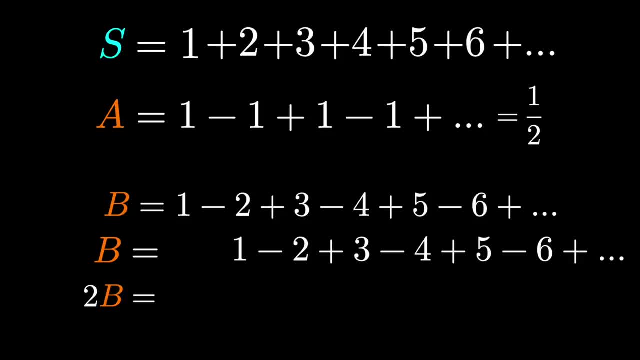 On the left, b plus b is 2b. On the right we would have: 1 plus 0 is 1.. Minus 2 plus 1 is negative 1.. Plus 3 minus 2 is 1.. Minus 4 plus 3 is minus 1.. Plus 5 minus 4 is 1.. We're getting 1 minus 1 plus 1 minus 1.. That's a. 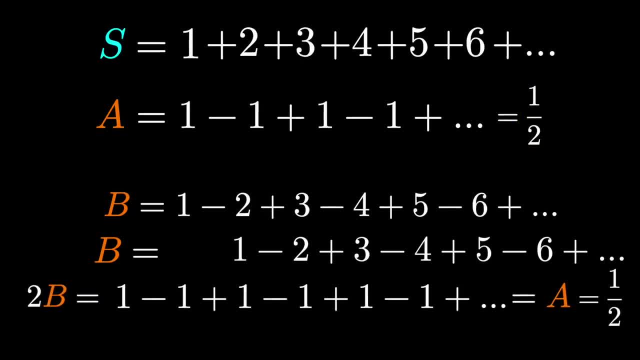 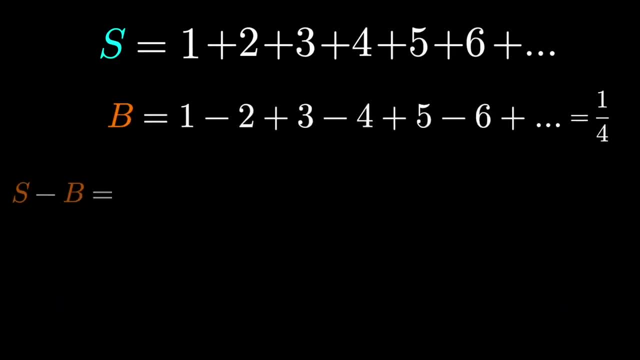 Which we said was 1 half. So 2b is 1 half or b is 1. fourth, Here comes the fun part. Are you ready? s minus b Line things up On the left is s minus b. On the right: 1 minus 1 is 0.. 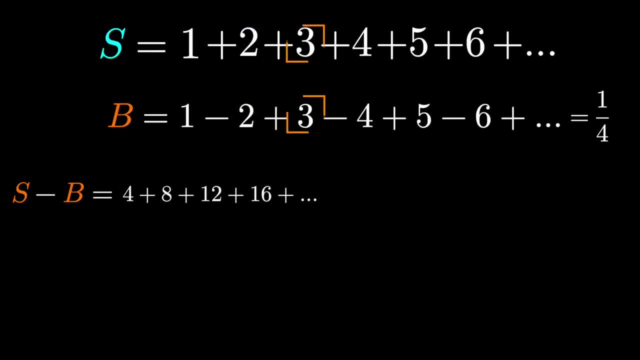 2 minus negative 2 is 4.. 3 minus 3 is 0.. 4 minus negative 4 is 8.. 5 minus 5 is 0.. 6 minus negative 6 is 12.. We're getting the pattern 4 plus 8 plus 12 plus 16 plus 20, on forever. 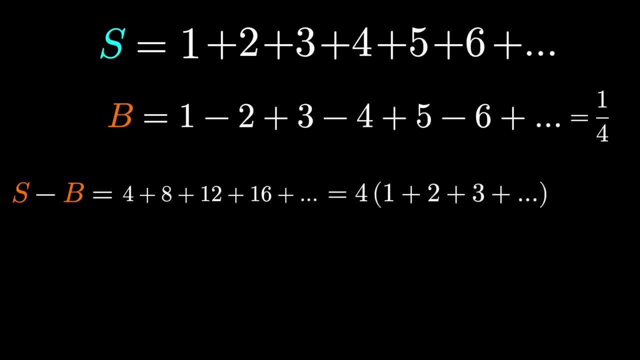 These all have a factor of 4.. We can factor a 4 out, So it's 4 times 1 plus 2 plus 3 plus 4 plus 5 on forever. That's what we called s. Then s minus b is 4s. We said b was 1. fourth, 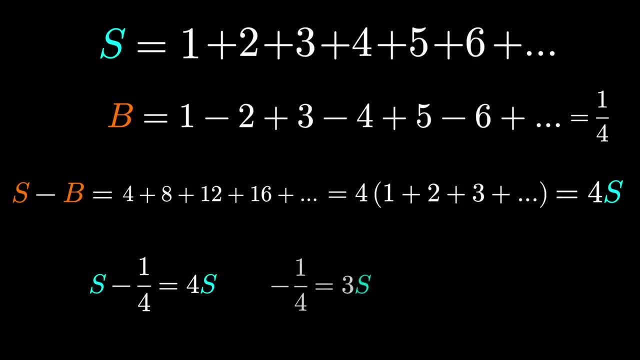 Just shuffle things around. So minus a fourth equals 3s, Or s is minus 1 over 12.. And so the sum of the natural numbers 1 plus 2 plus 3 plus 4 on forever is minus 1 twelfth, And I'm sure you're fairly skeptical of this, but there's certainly plenty. 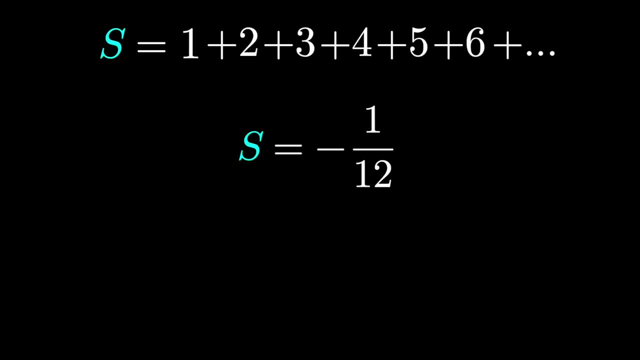 of info online and on YouTube pointing to this result. What's going on with this argument? here, Whether you realized it or not, we kind of bent the rules of algebra. I mean, who says that The distributive law works over an infinite sum? like this? We typically only assume the distributive. 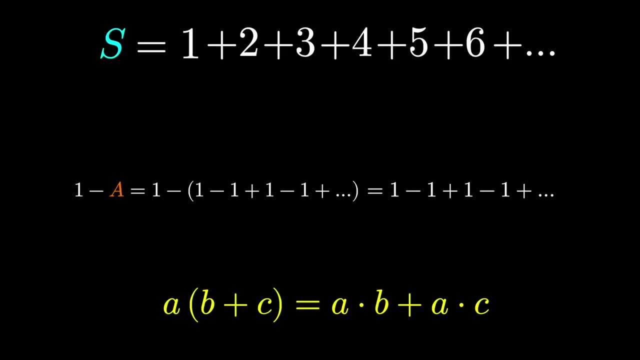 law holds for finite terms. Now maybe you think the distributive law should indeed hold for infinitely many terms, and maybe you're right. Whenever we deal with algebra, the regular distributive law is taken as an assumption. It's called an axiom. You can't prove the distributive 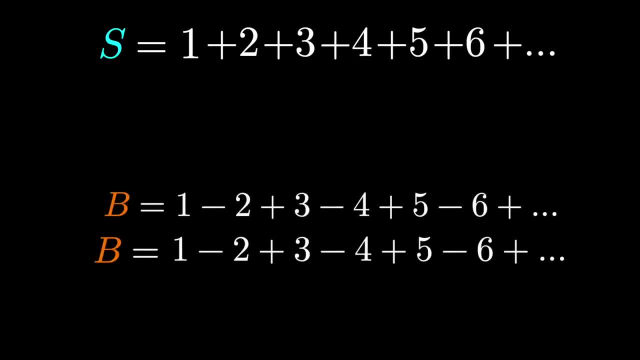 law. The other issue is there's also some business with how we're grouping the terms when we're adding. You see, the distributive law works over an infinite sum like this. We typically only assume the works for finite sums, but does it work for infinite sums For math to work? we 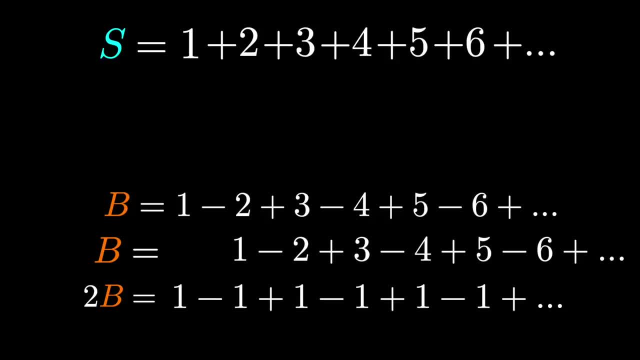 all need to agree on a set of rules, axioms to follow and then deal with the consequences. But the big problem here is that if you want to accept these rules like an infinite distributive law, you have to accept those consequences. and applying these same rules can also lead us to different results, which I'll show. 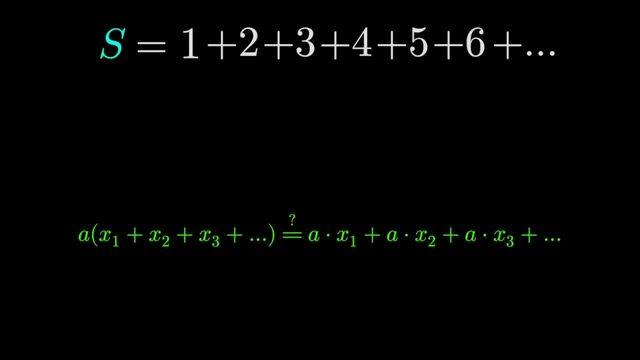 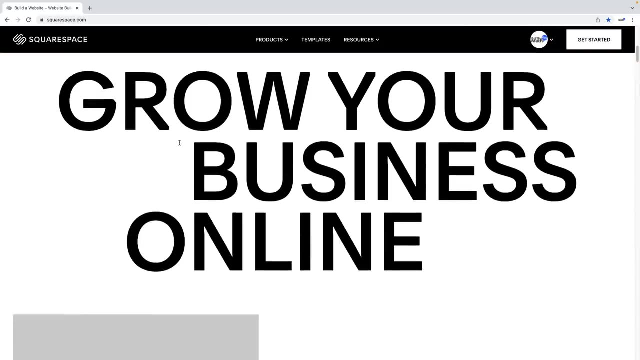 you. But while we're speaking of making up your own rules and being creative, you should check out the sponsor of today's video: Squarespace. Squarespace makes it easy for creators and educators to share or monetize their content. There's everything you could need from collecting donations or payments. 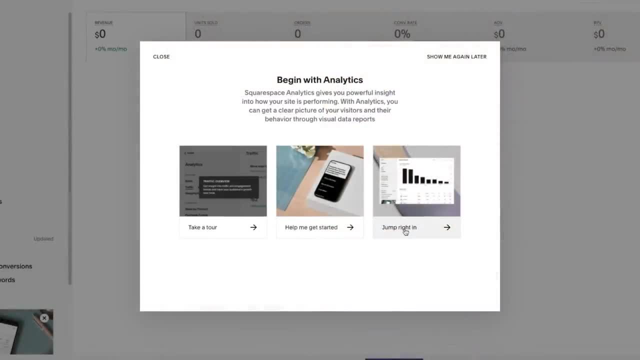 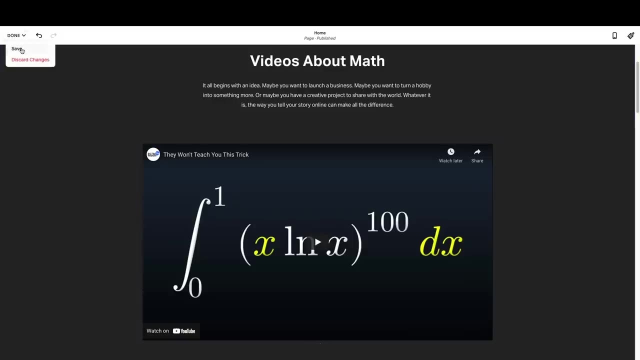 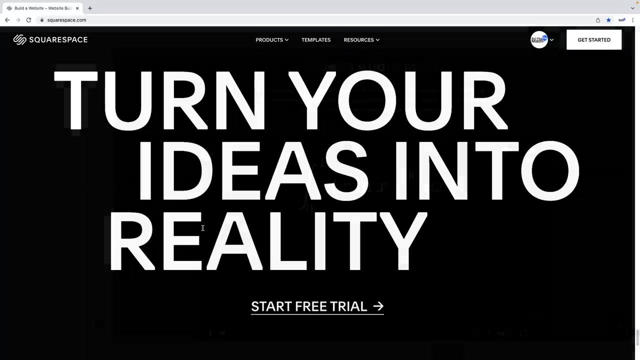 building email campaigns and powerful analytic tools to gain insights. I recently rebuilt my site with Squarespace and it's much more intuitive and clean than other platforms I've tried. I think it just looks a ton better and way more professional too. There's no risk to try it out, since you 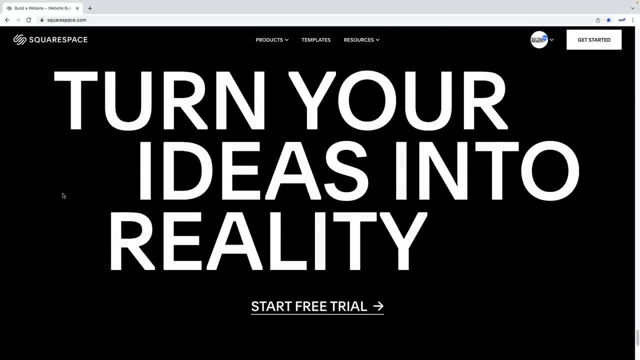 can head to Squarespacecom for a free trial and, when you're ready to launch, click the link in the description of this video to save 10% off your first purchase of a website or domain. Let's look at our value S from a different 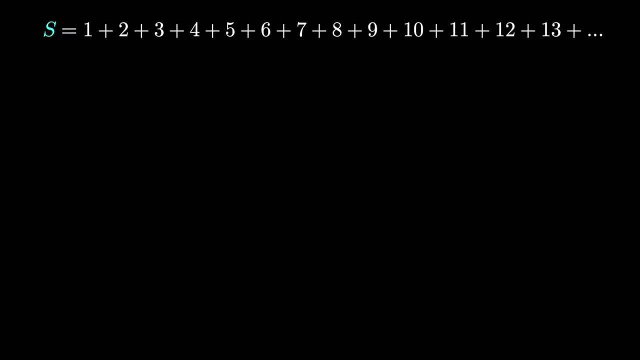 point of view. I've written out our sum, just with more terms. It still goes on forever. I'm gonna leave the first 1 and then look at the next three terms: 2 plus 3 plus 4, that's 9.. Look at the next three terms: 5 plus 6 plus 7, that's 18.. The 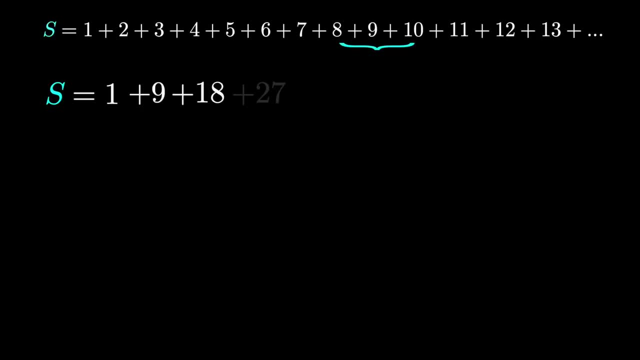 next three terms: 8 plus 9 plus 10 is 27.. We can write this by grouping three consecutive terms as 1 plus multiples of 9.. In fact, we can factor out that 9 from all of those terms, so it's 1 plus 9 times. 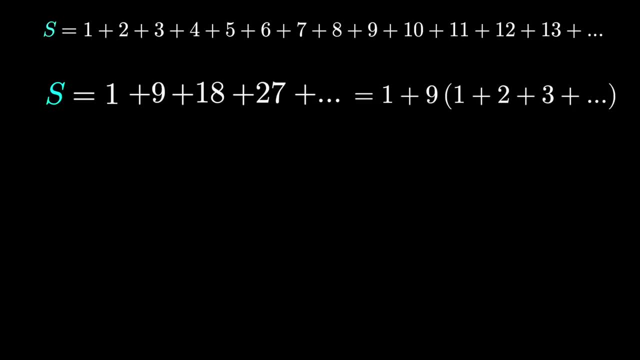 1 plus 2 plus 3 plus 4, on forever. Well, that's S. So 1 plus 9, S is S, 1 is minus 8 S, or S is minus 1 eighth. And so this method tells us that the sum of the 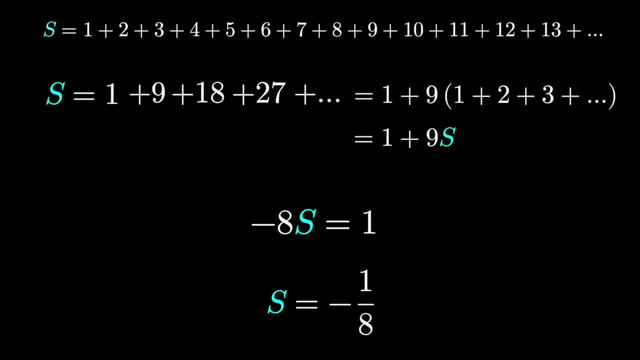 natural numbers is negative 1 eighth, And we found this result using the same infinite distributive law we used before. So which is it? Is it minus an eighth or is it minus a twelfth? Maybe this infinite distributive law isn't a good rule to hold on to, But I hear you say: wait, in my calculus class. 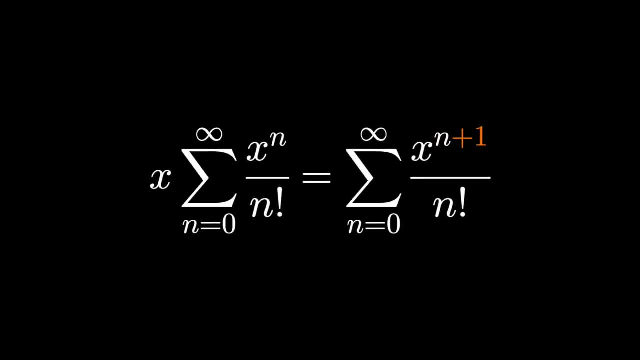 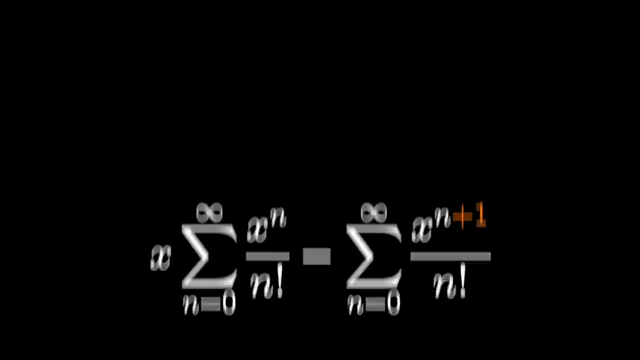 I used an infinite distributive law. all the time We factored and distributed things in infinite series And fair enough, But those were probably convergent series. They summed to a finite value using traditional methods in calculus. Even just using the very first test you learn in calculus for determining if a series diverges, it's: 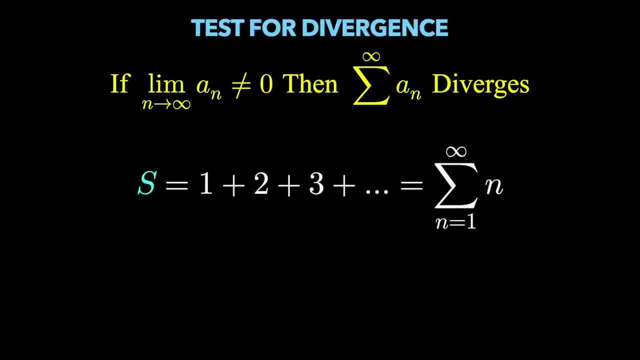 just called the test for divergence, we immediately see that this series in question indeed diverges. You just take this limit as n goes to infinity, you get infinity, which isn't zero, Meaning the sum of the natural numbers is a divergent series. We can't use this infinite distributive law on it, But the